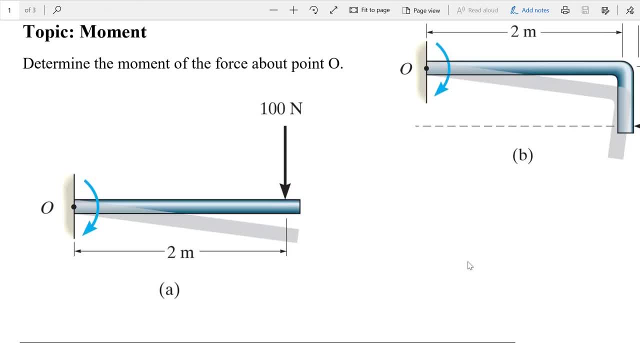 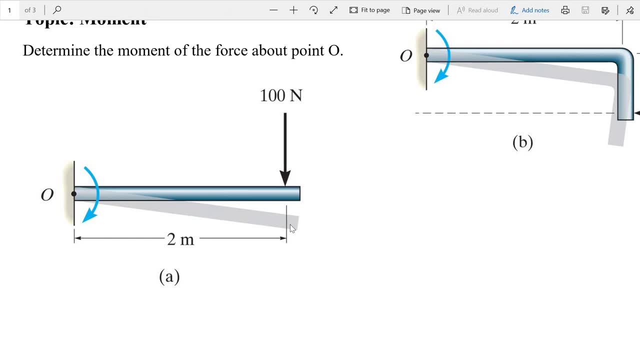 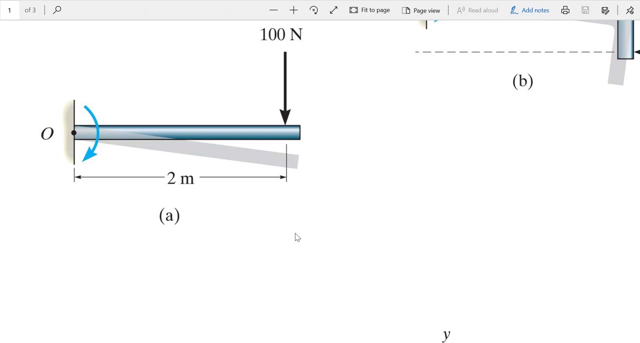 hello everyone. we are going to solve a couple examples for 2d moment. so determine the moment of the force about point O. so in this problem you have a force, 100 Newton, and you want to find the moment about point O. so the moment about O should be the force times the perpendicular distance. but this force is 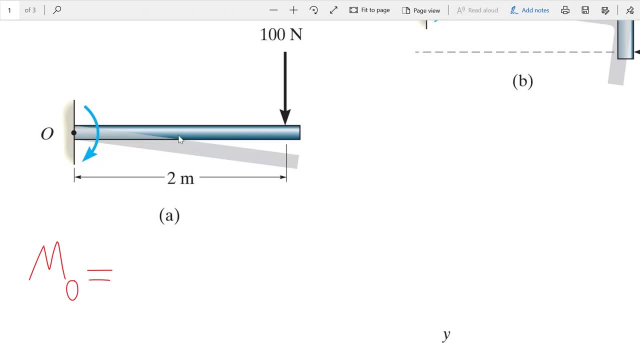 creating the clockwise rotation is pushing a member to rotate clockwise and we said that the clockwise convention would be negative. force is 100, the moment arm is 2, the perpendicular distance, so I have negative 200 and the unit for moment is Newton meter. Newton meter, let's go to. 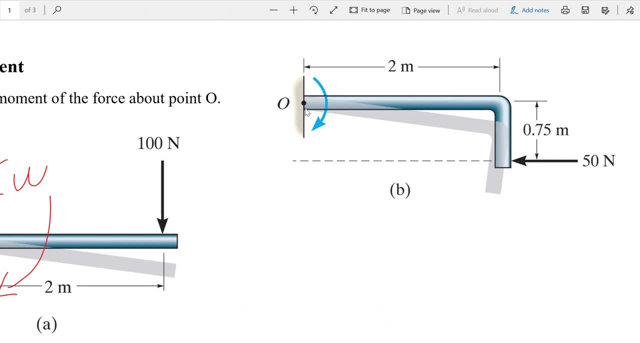 the another problem. you want to find a moment about point O. here again, this force is forcing the member to rotate clockwise, so my moment would be negative. that's how I determine the sign of the moment here. this shadow shows the rotation of our part. what is the force is 15 years, but what is the moment? arm. 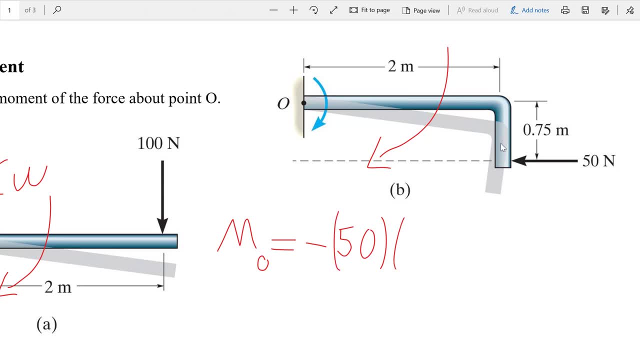 we have multiple dimensions, but remember we always deal with the perpendicular distance and that would be 0.75 meter. it really doesn't matter how far is this lens: 0.75, the result would be negative. thirty seven point five. the unit again is Newton meter. 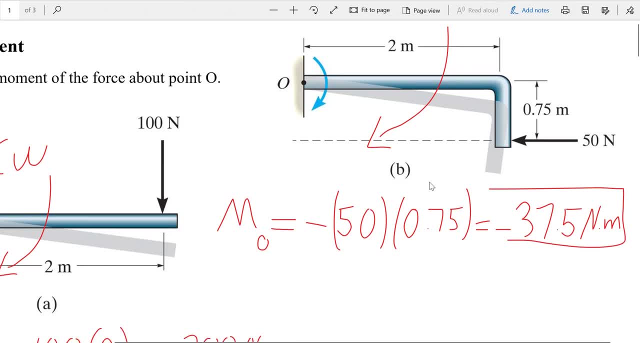 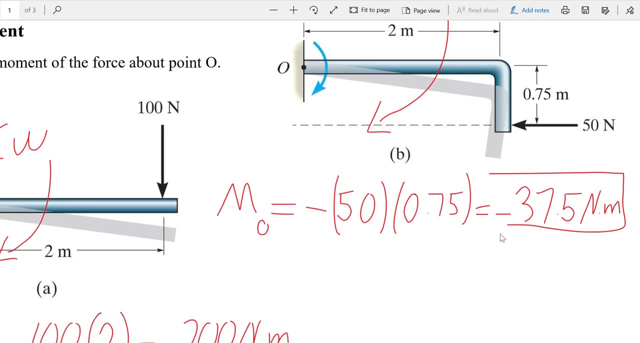 well, our convention is. positive would be counterclockwise and negative clockwise. sometimes a negative counterclockwise is also reported as thirty seven point five Newton meter clockwise. so instead of saying negative reporting, negative to show the clockwise, you just write it here: clockwise. both convention is is common. 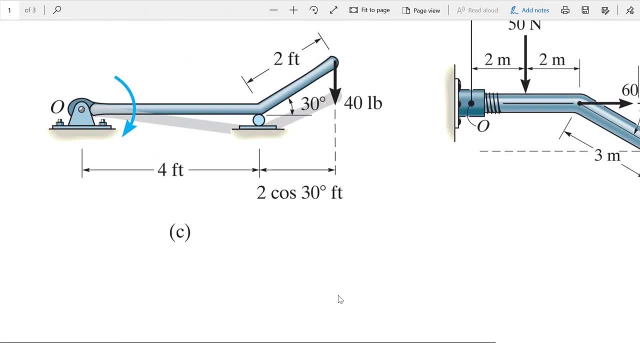 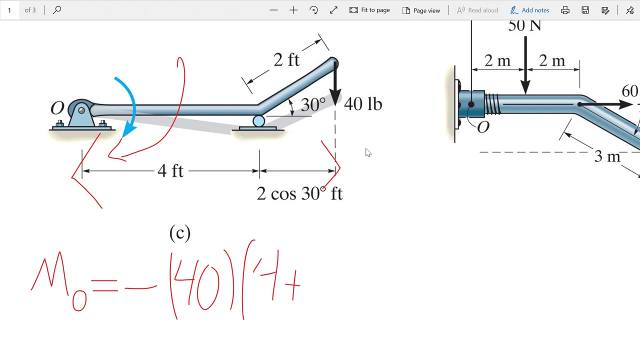 so let's look at another problem here, going to find a moment about trying to find the moment. point 0 again is rotating, a member clockwise negative. the magnitude of the force is forty. remember beloenity expelled a moment are we need to find a perpendicular distance. so that would be the total distance here, which is 4 plus 2 cosine. 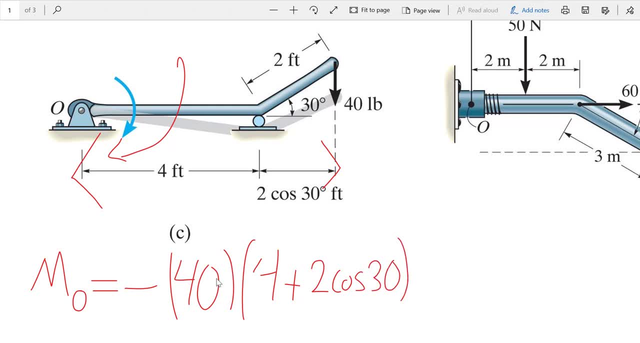 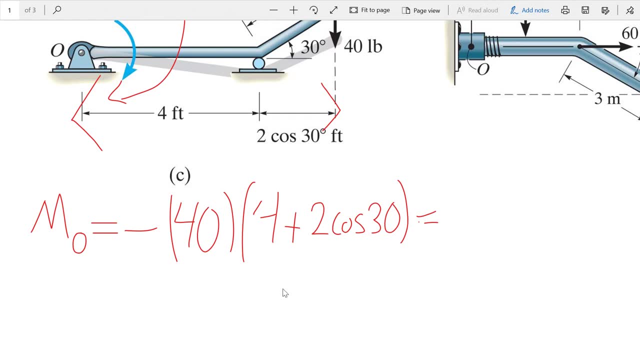 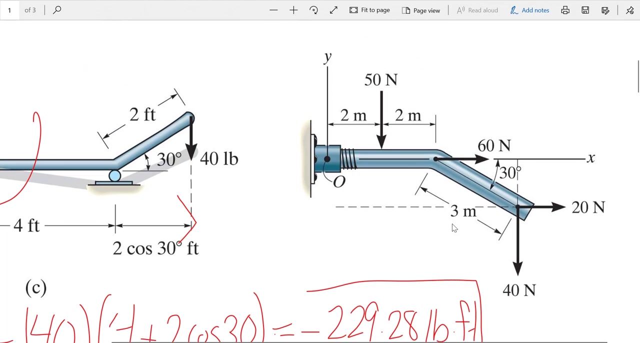 30, the fourth times the moment R, therefore our MO, or the moment about point O, would be negative 229.28. and remember, the unit system here is pound feet and this negative signs indicate clockwise. let's look at this problem now. here in this image we have multiple forces. I'm going to find the 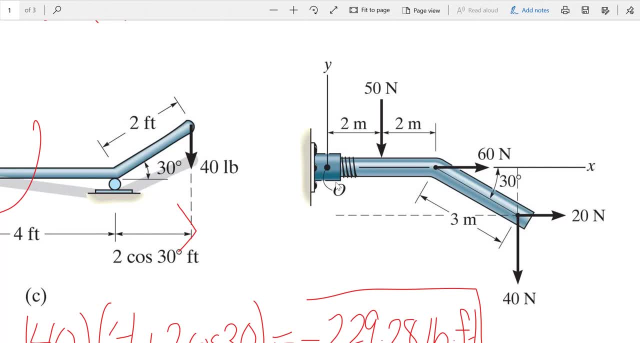 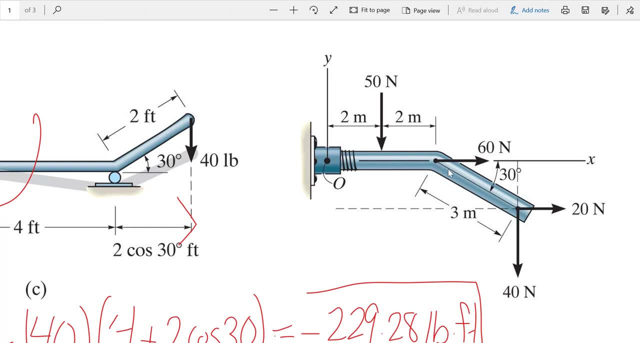 moment of all forces about point O. we have one, two, three, four, but not all of them are creating a moment about point O. if you look at the image, we see that this 60 Newton is going through point O and is not causing our member to rotate, or in other words, the moment arm is zero. so 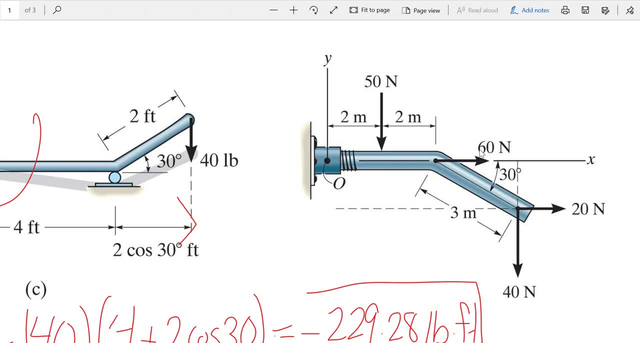 this, 60 Newton is not creating any moment for us. we can include it into a equation, but we need to multiply it by zero, which will remove this term. our force is 50 Newton is creating a moment and the moment arm is 2 meter is creating a. 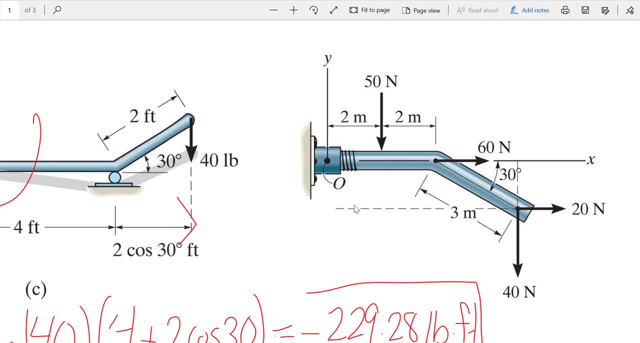 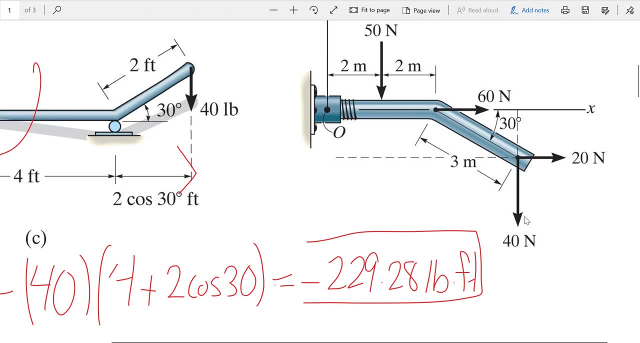 member, creating a member to rotate, causing a member to rotate clockwise, so that will create a negative moment here. these two forces, we have 20 Newton. the moment arm for this 20 Newton force is from here to here and it's creating, causing our member to rotate, counterclockwise. so this force is